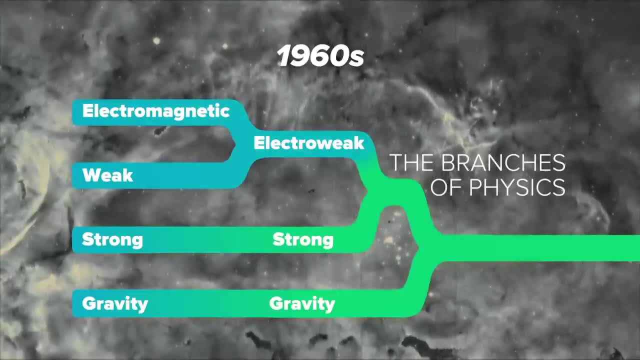 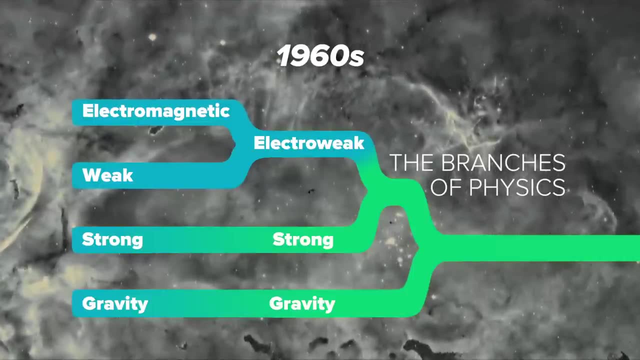 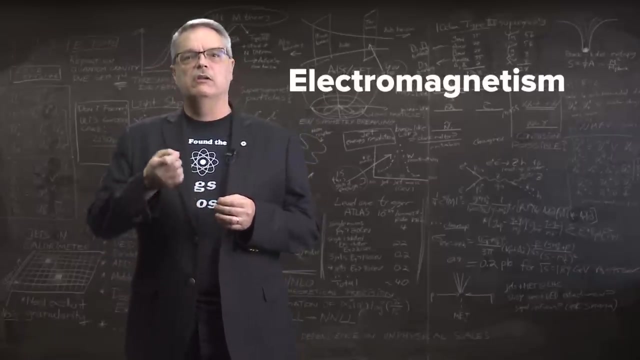 theoretical physicists were able to show that they could unify the weak nuclear force and electromagnetism. Now that turned out to be a surprising thing, for a couple of reasons. The electromagnetic force behaves similar to gravity. It is a force with an infinite range which weakens as the square of the distance between two charged objects. That's. 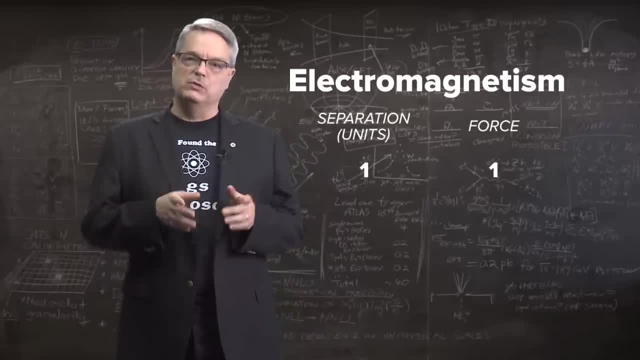 just mathematical fancy talk for saying that if you double the distance between two objects, the force between them drops by 2 squared or 4.. If you triple the distance between them, the force drops as 3 squared or 9.. In contrast, the Higgs boson is a very complex object. It is a very complex object, It is. 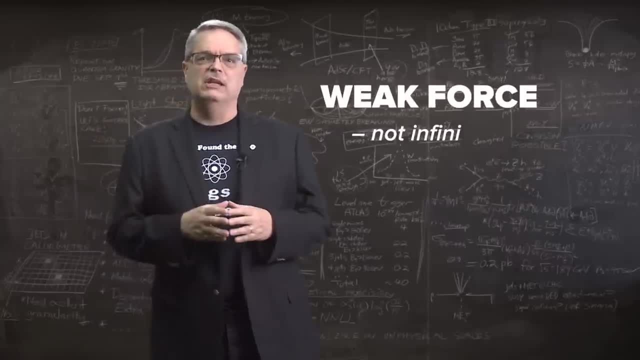 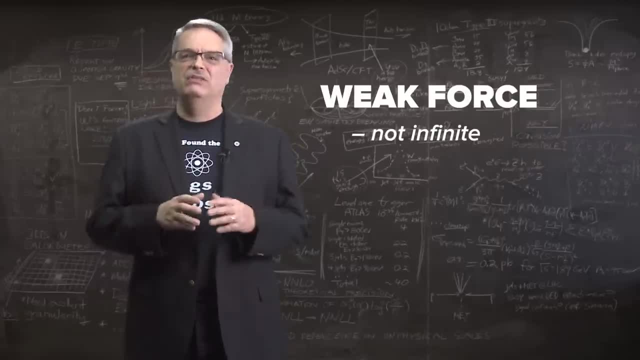 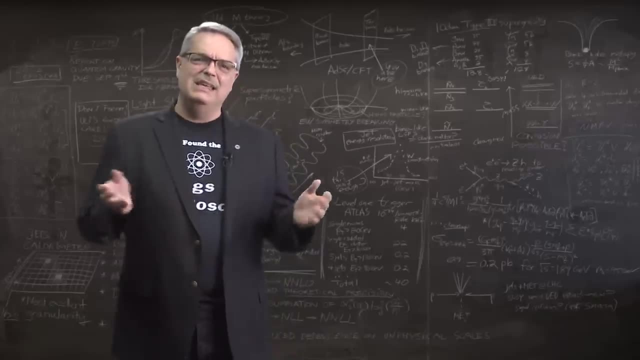 one-thousandth that of a proton, but then doesn't have any real effect after that. Yet scientists were saying that these two forces were the same thing. That didn't make any sense until the Higgs field was invented. The Higgs field is kind of like a Band Aid. 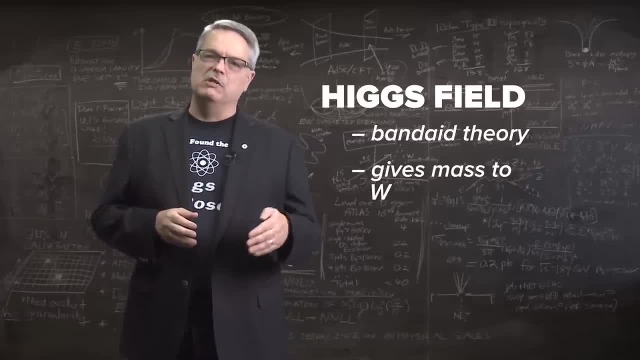 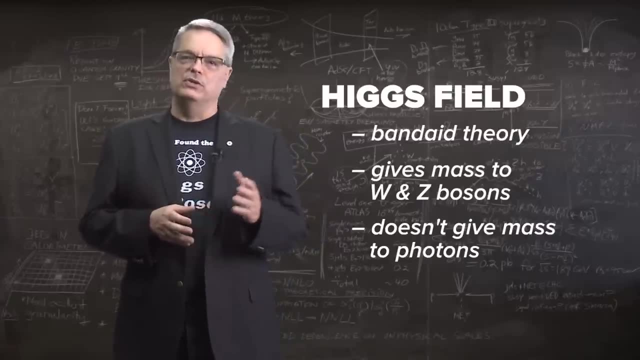 theory that was added on. It gave mass to the particles that transmit the weak force and didn't give mass to the particle that transmits electromagnetic force. The name of the weak force particles are the W and Z bosons, while the name of the particle 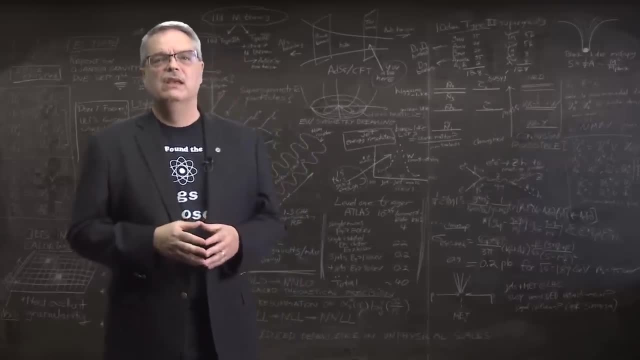 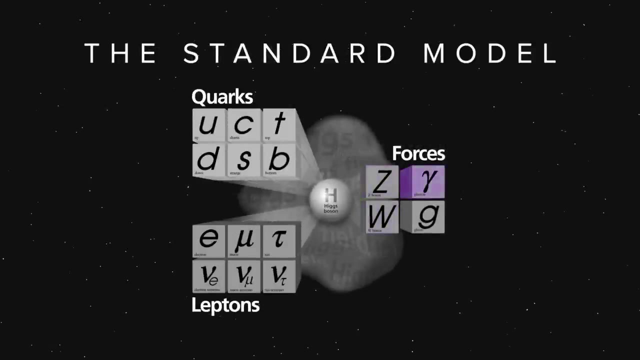 that causes electromagnetism is the photon. So that's how the Higgs field originally fit into the theory. It gave mass to the W and Z bosons and not to the photon, which is also a boson. But there are other particles in the Standard Model, specifically the quarks and leptons. 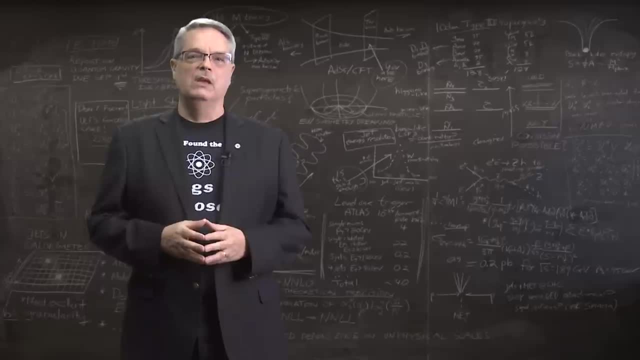 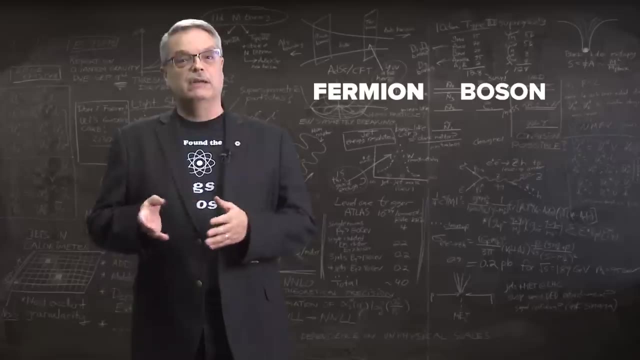 which are the particles that actually make up matter. Quarks and leptons are fermions, not bosons. The difference between a fermion and a boson is that fermions have a different amount of spin compared to bosons. The fermions have a spin of a half, three halves, five halves and so on, while the 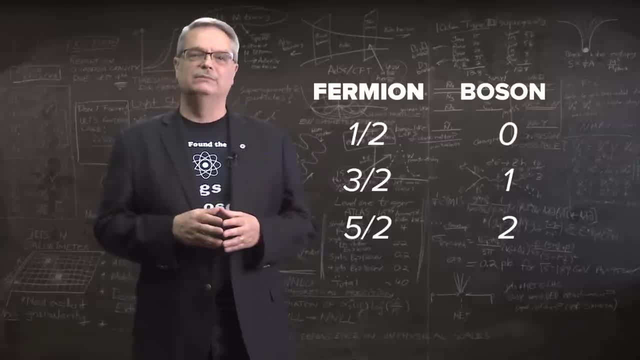 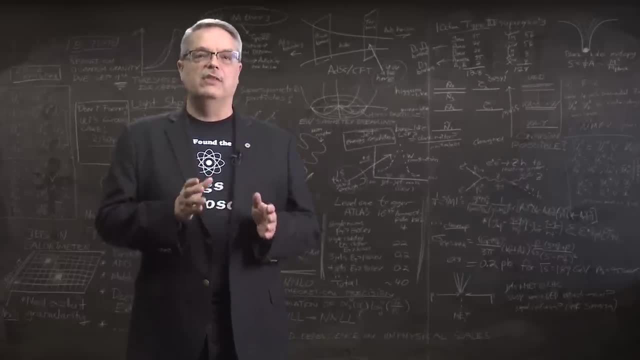 bosons have a spin of zero, one, two, etc. I'll talk more about the significance of the differences of fermions and bosons in a future video, but the bottom line is that they are different and the original Higgs theory only gave masses to bosons. 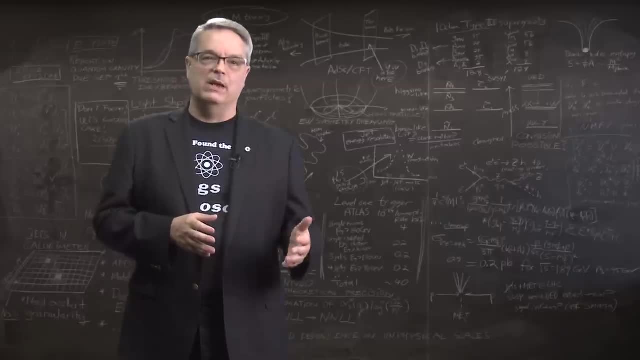 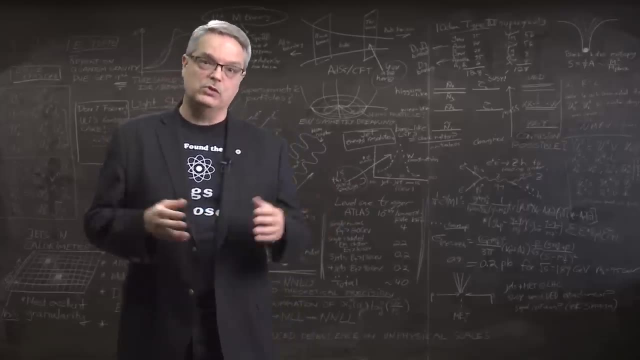 But it would sure be economic If the Higgs field would also give mass to the fermions. It doesn't have to be that way. The mass of fermions and the heavy bosons could have gotten their mass from different sources. So a very important test was to see if the fermions also got their mass from the Higgs. 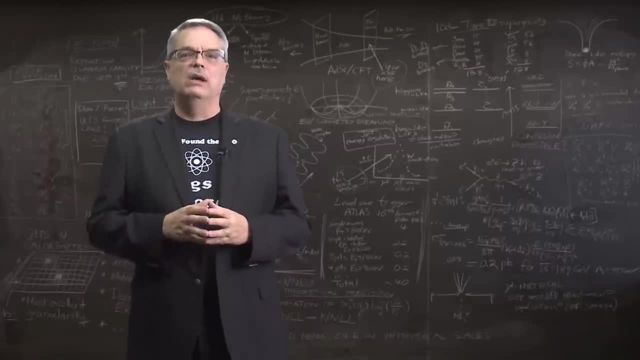 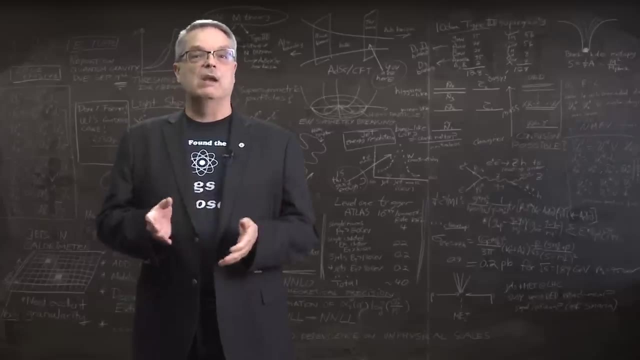 field. So how would you do that? Well, to do that, you have to remember a very crucial point. You often hear people say that the Higgs bosons interact more with heavy particles, And that's true, But there's a better way to say this. The correct way to say it is that the particles that interact more with the Higgs field and boson get more mass. This is a very subtle point, so I'll say it again: It's not that heavy particles interact more with the Higgs field. 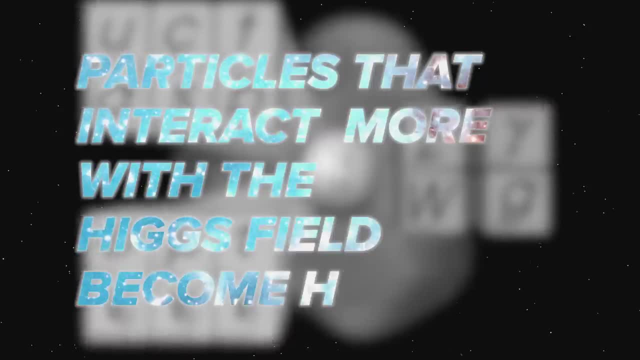 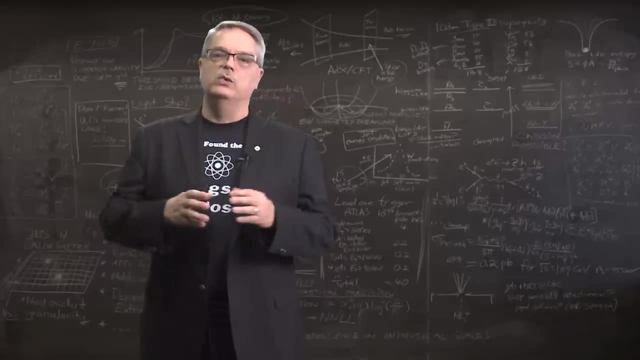 It's that particles that interact more with the Higgs field become heavy. It's the interaction with the field that comes first, and the mass is the consequence. So how can we test this, Given this connection between the mass of the particles and the degree to which they're 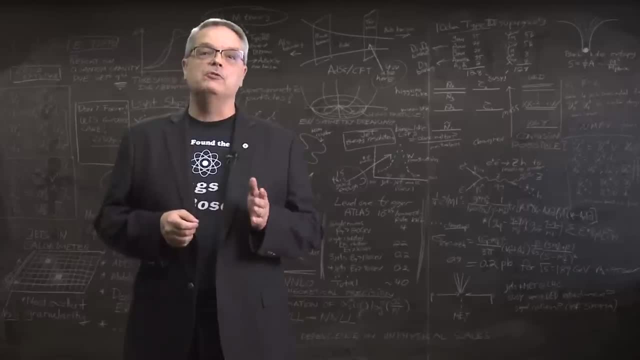 burning and the degree to which the Higgs field interacts with them. we can predict into which particles the Higgs boson prefers to decay and which it doesn't, And remember that we can measure the mass of the particles without knowing anything about the Higgs boson at all. 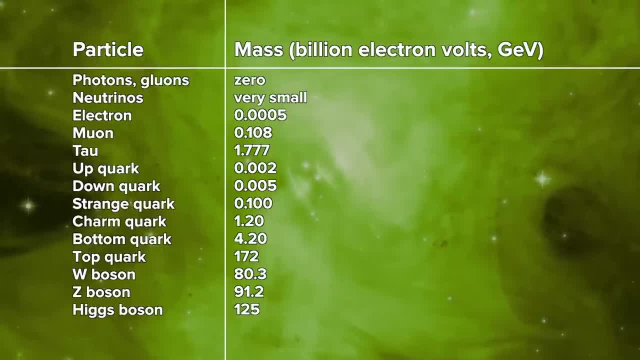 We've been doing that for decades. We see here the mass of all of the known subatomic fermions. The electron has a mass of 0.0005 billion electronvolts, while the top quark is the king of the subatomic world. 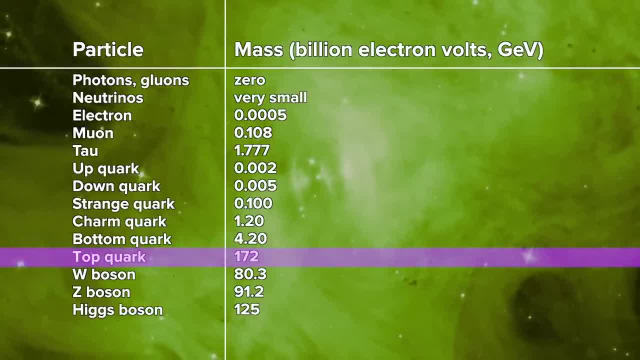 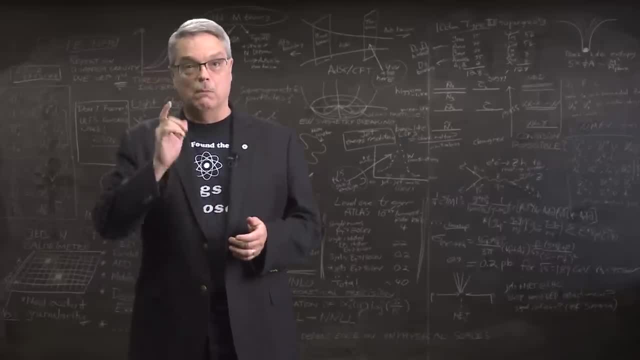 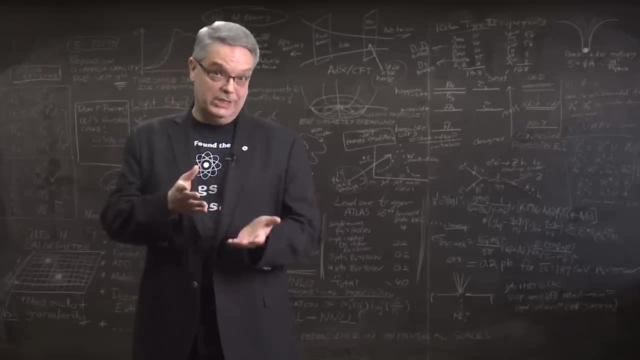 with a mass of 172 billion electron volts, and the other particles are somewhere in between. If we assume that the mass of the fermions and bosons are both caused by their interaction with the Higgs field, we can use that theory to predict how often the Higgs bosons will. 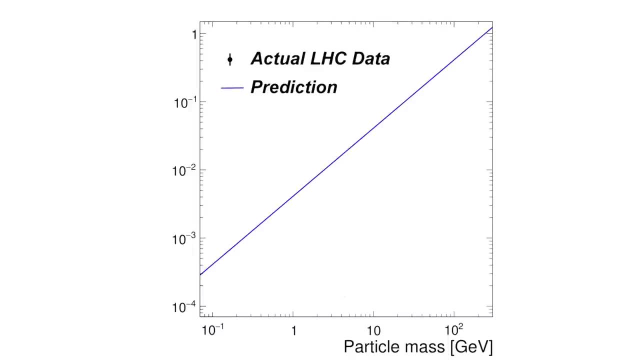 decay into those particles, And the prediction is shown here on this graph. If the Higgs theory is right for both fermions and bosons, the data for each particle should appear exactly on this line. So let's take a look, shall we? 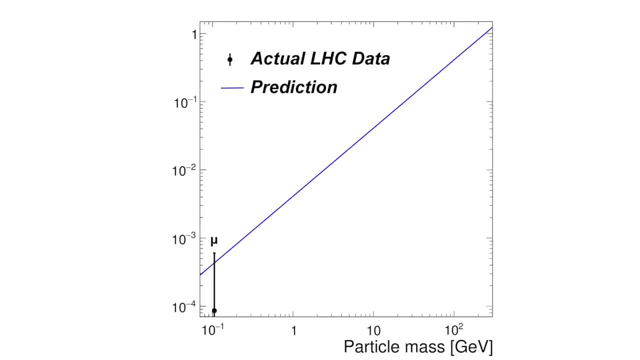 Okay, so what happens when we add the data for the muon? Well, the black circle is the actual measurement, but the vertical line is the uncertainty on the measurement. and as long as the black line crosses the prediction- or at least comes, 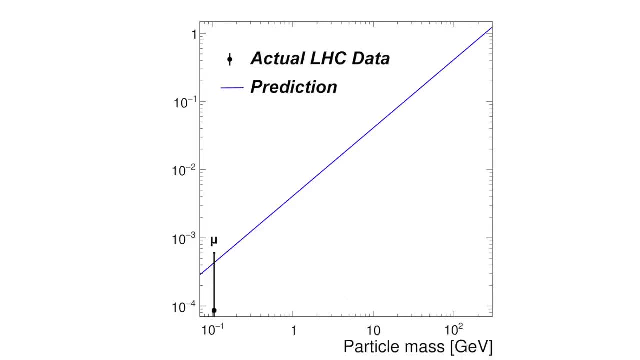 very close. we can call that an agreement. So the muon measurement agrees with theory, although the uncertainty is pretty big. What about the tau lepton, which has a mass of 1.8 billion electron volts? How do Higgs bosons decaying in the muon measure? 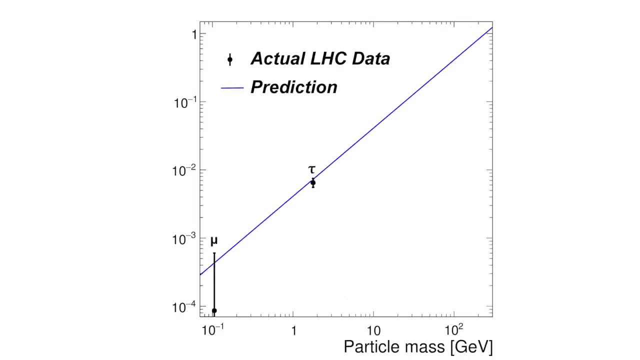 And the tau lepton's work, We see that the measurement agrees with the prediction pretty well. What about the bottom quark, with a mass of about 4.2 billion electron volts? We see pretty good agreement, although the error bar doesn't quite cross the prediction. 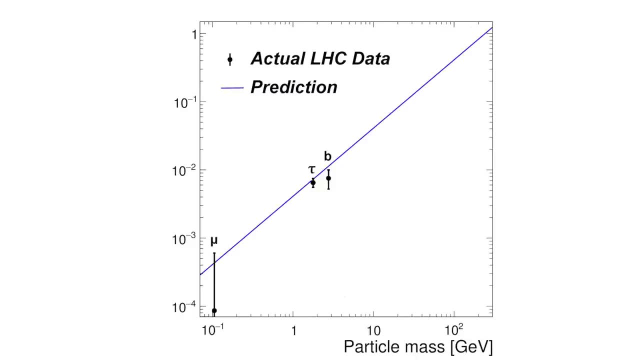 But it's close and this is real data, so that's considered reasonable agreement. And when we add the heavyweight top quark with its mass of 172 billion electron volts, we see again: pretty good agreement. So far, so good. Now what about when we add the heavy bosons? 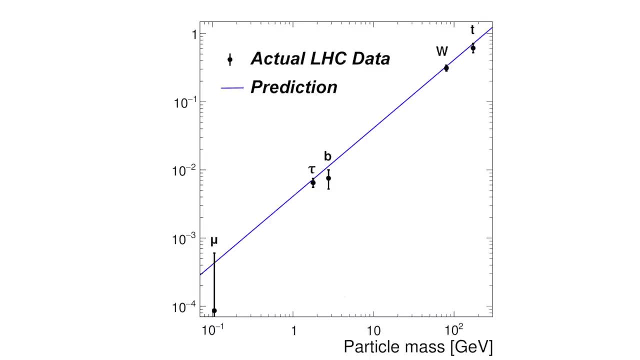 What sort of agreement do we see there? The W boson has a mass of 80 billion electron volts and we see that it plops right on the line. And finally we add the Z boson with a mass of 91 billion electron volts. 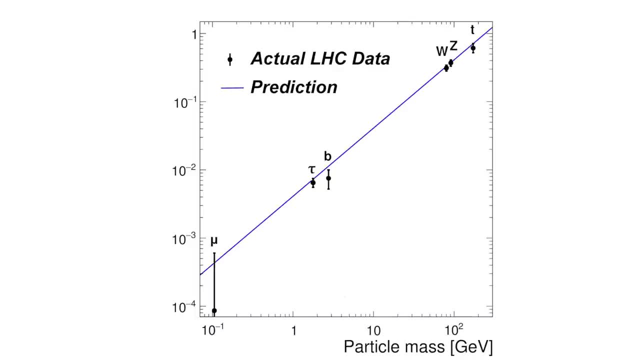 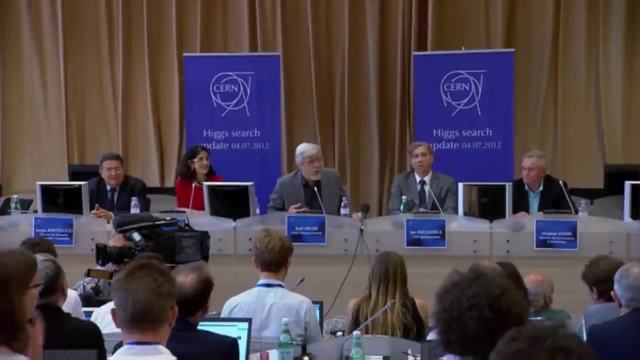 We see that this also agrees with prediction, So this is really extremely impressive support for the idea that the particle discovered back in 2012 is really the Higgs boson predicted back in 1964.. On the other hand, that means we aren't exactly sure what to do next. 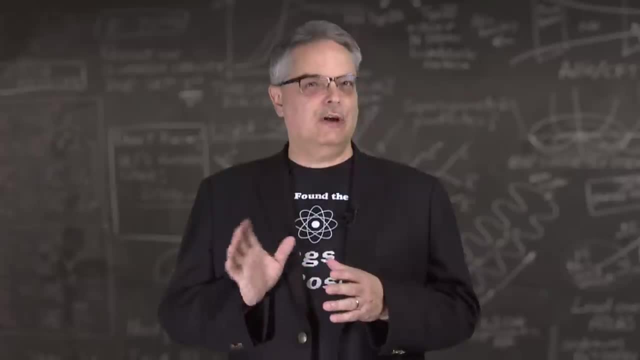 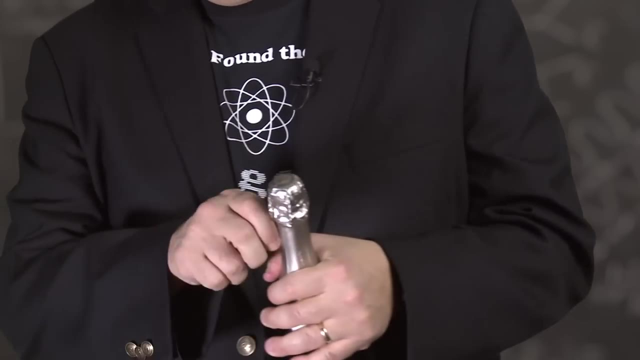 While a success like this needs to be celebrated in some ways, it would have been far more interesting to see some real discrepancies between the prediction and the data. But the universe isn't obliged to give us surprising results. We scientists must accept the truth, whatever that may be. 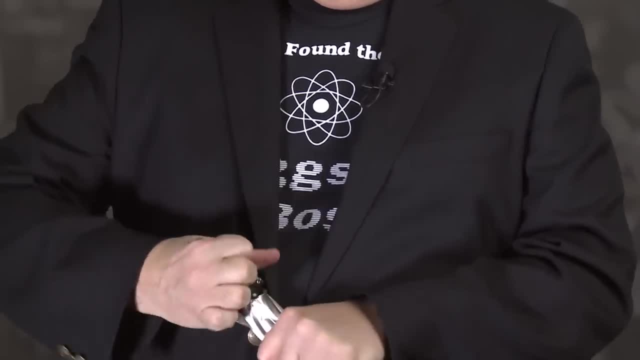 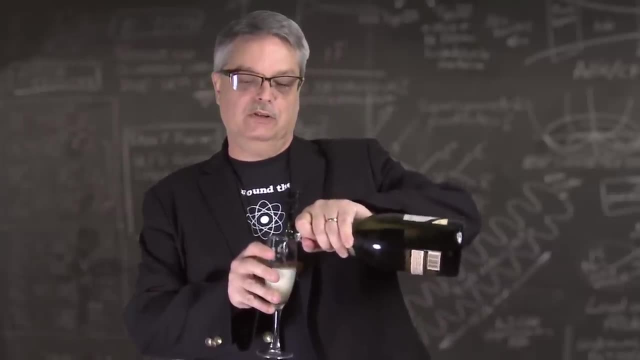 So we'll keep looking into the data, hoping to find the next clue, But in the meantime, I'd like to propose a toast for all of my colleagues on the ATLAS and the CMS experiment, As well as the amazing LHC operators for a measurement that's absolutely astounding. Cheers.